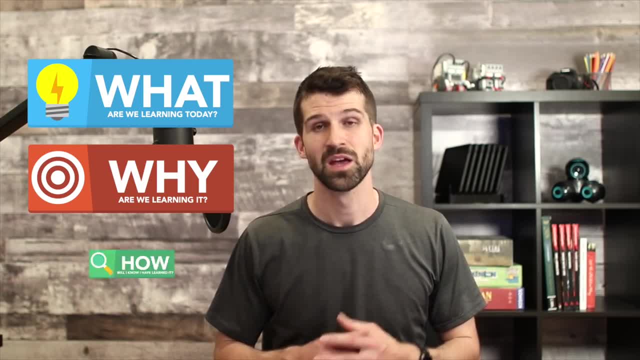 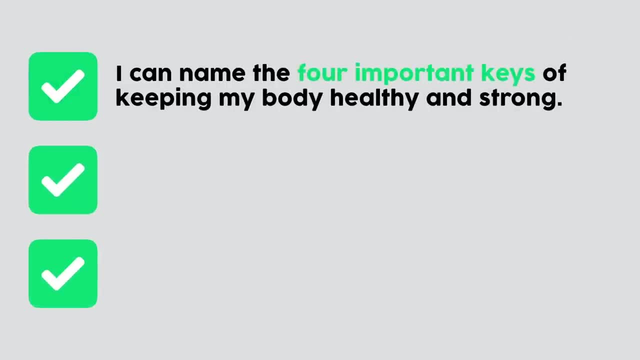 us feel good and be able to take care of the people around us. So your learning targets for today's lesson are as follows: I can list the four important keys of keeping my body healthy and strong. I can explain how physical activity helps keep my body healthy and strong. 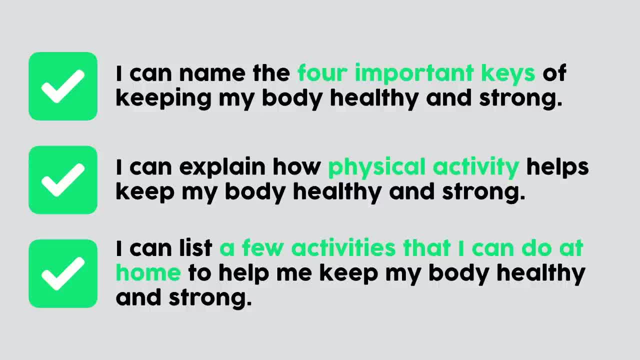 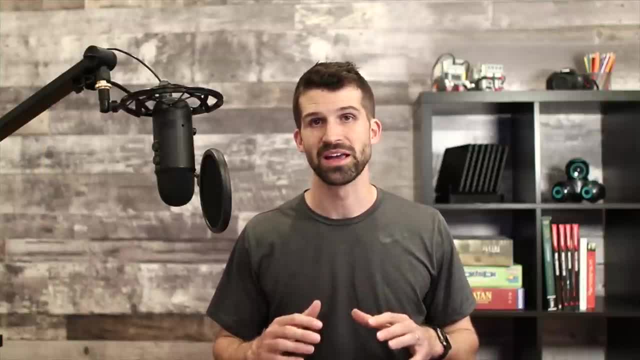 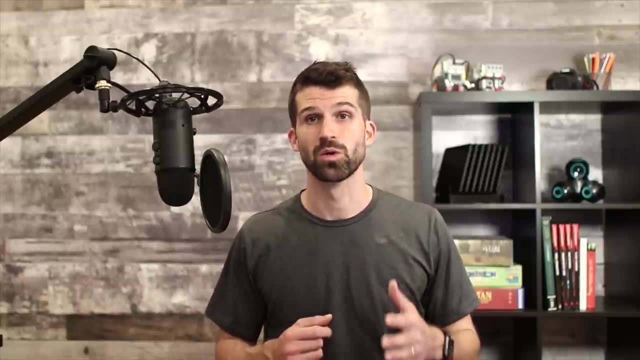 And I can list a few activities that I can do at home to help me keep my body healthy and strong. So remember that learning is a journey and everybody learns at their own best, But one of the best things you can do in order to be a successful learner is to set a goal. 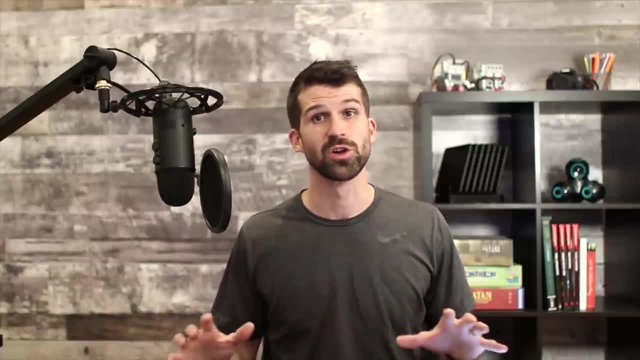 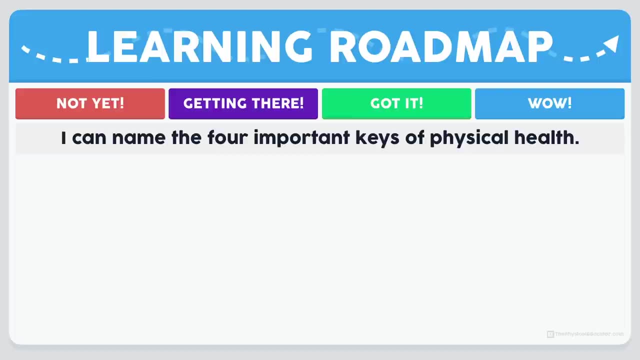 for your learning. So, that being said, let's take a peek at our learning roadmap for today and try and figure out where we're currently at in our learning. So the roadmap for today's learning looks like this: If you're at the not yet level, that means you don't know any. 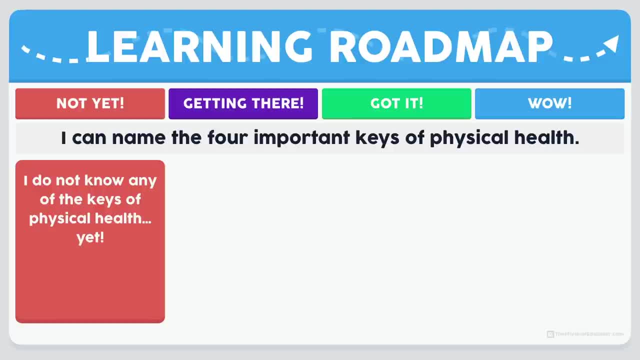 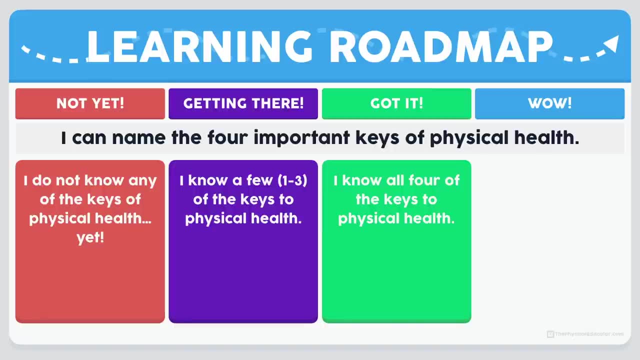 of the keys to physical health. At the getting there level it means that you know a few- so one to three- of the keys to physical health. And at the got it, it means that you can name all of the keys of physical health. But if you're 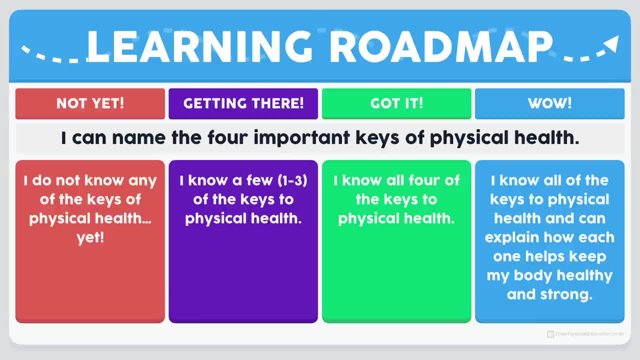 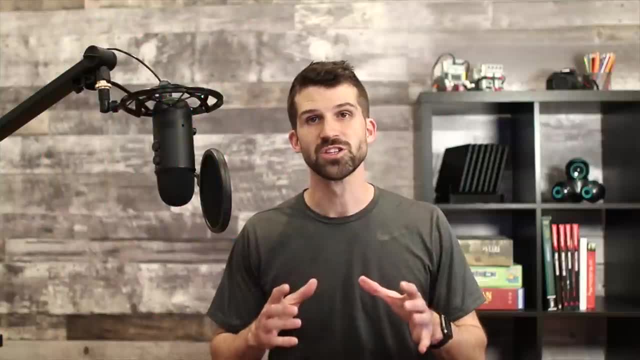 at that wow level. not only do you know all the keys of physical health, but you can also explain in your own words how each one helps keep your body healthy and strong. So what I want you to do is to look at that roadmap and try and reflect where you're currently. 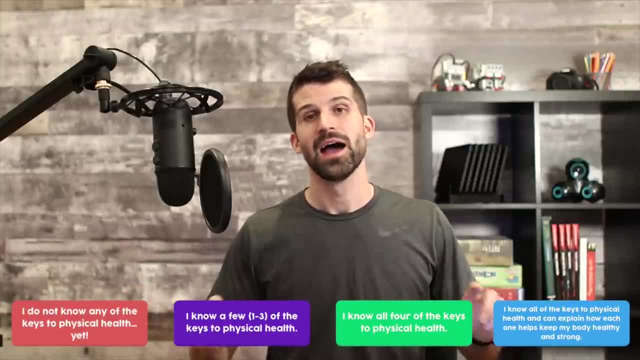 at in your learning. Go ahead, I'm going to put it right down here for you, And when you figure out where you're at in your learning right now, what I want you to do is I want you to say it out loud. 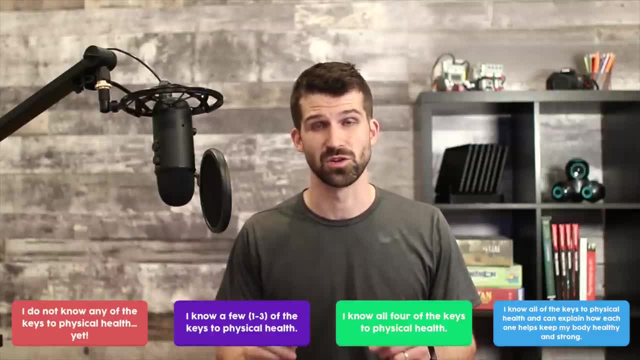 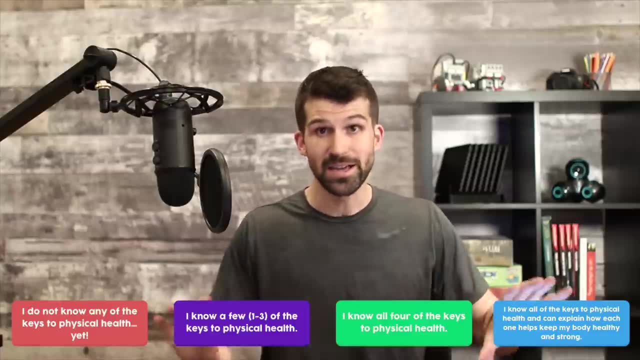 I want you to say what your goal is now for your next step in your learning. What do you need to achieve next in order to keep making progress as a learner? So go ahead, take a peek, and I want you to say out loud: You're at home so you can be as loud as you want. 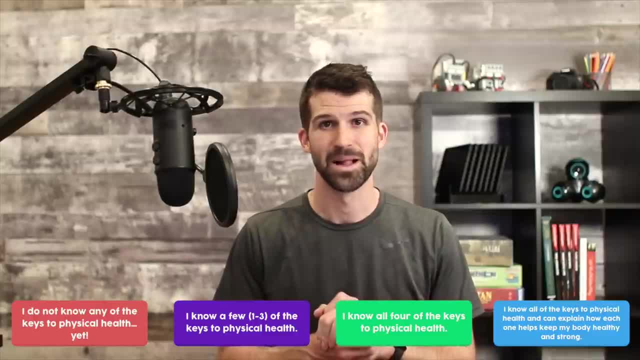 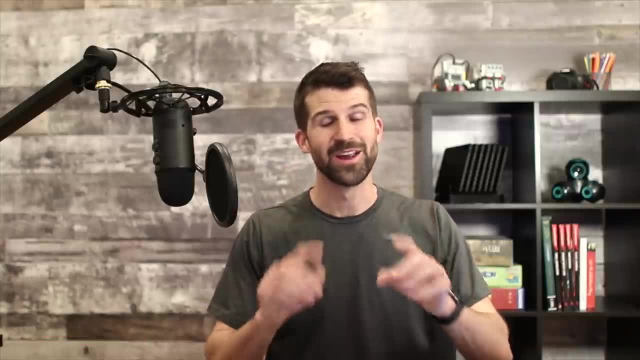 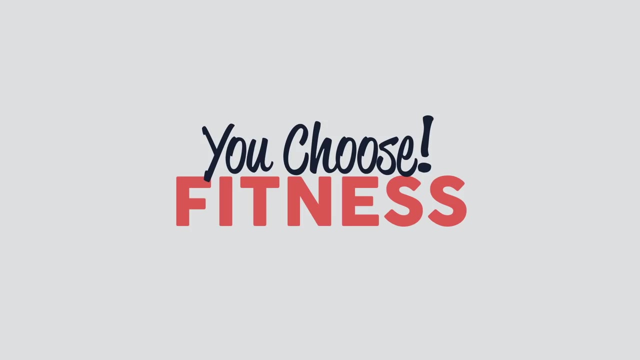 right now, I'll just wait right here. All right, you got it Okay. so, with that goal in mind, with our target set, let's get moving. All right. so the first thing I want you to do is to make sure that you have enough free. 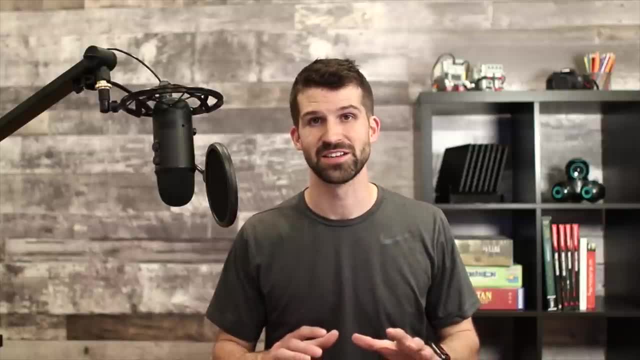 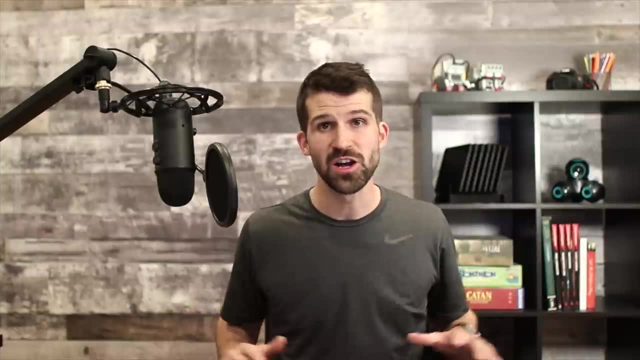 space around you. You don't need a ton of space for today's activities, But I do want to make sure that you're not going to accidentally knock over anything breakable and get yourself in trouble. So just make sure you've got enough space And, once you do, before we start our 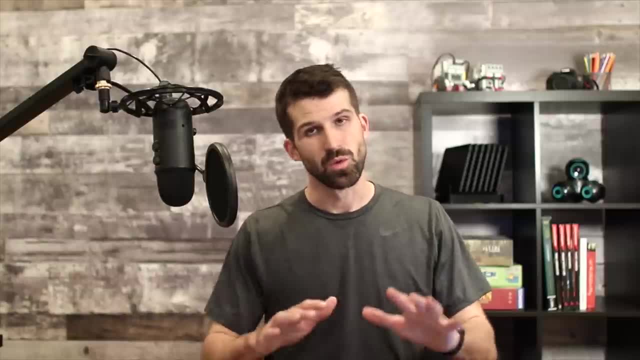 warm up. we're just going to take a mindful moment, So I want you to sit down on the ground, nice and calm, crisscross applesauce. I want you to close your eyes And I want you to put one hand on your chest. 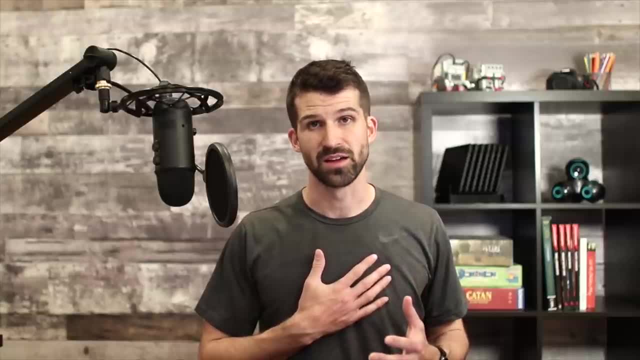 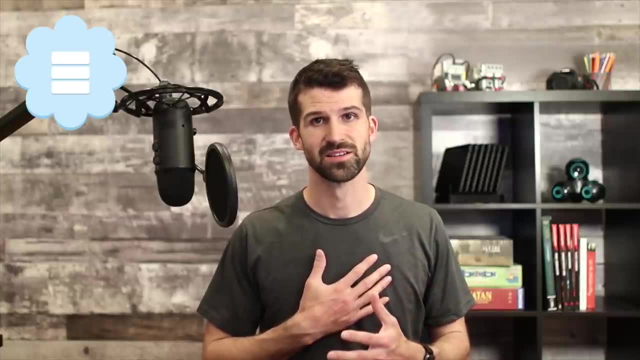 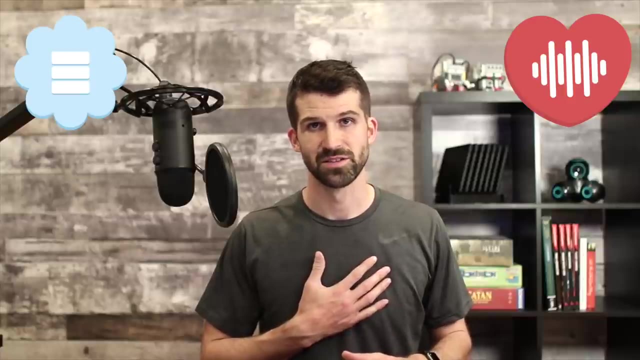 And here's what I want you to notice: Notice your breathing. Is it deep Or is it shallow? Is it slow Or is it fast? What about your heartbeat? Is it beating really hard Or is it beating nice and soft? Is it beating really slow Or is it beating really fast? What about? 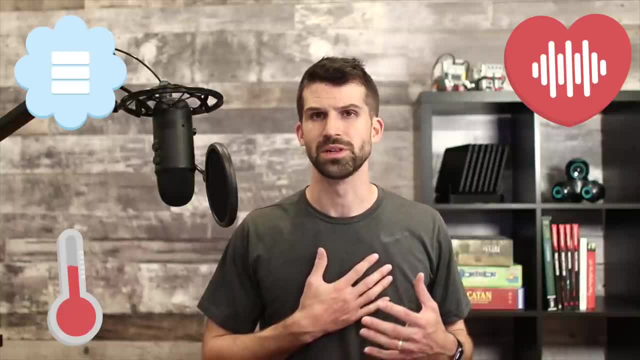 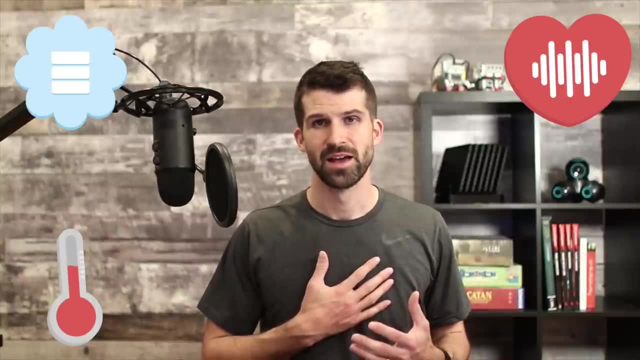 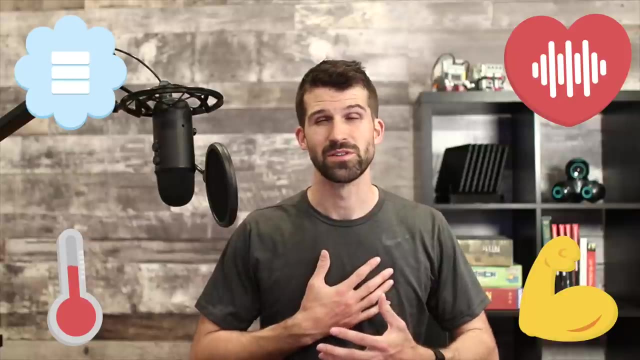 your body temperature right now. How do you feel? Are you really warm Or are you cool? Do you feel yourself sweaty Or is your brow nice and dry? And what about your muscles? How do they feel? Do they feel tight Or do they feel loose? Do they feel cold Or do? 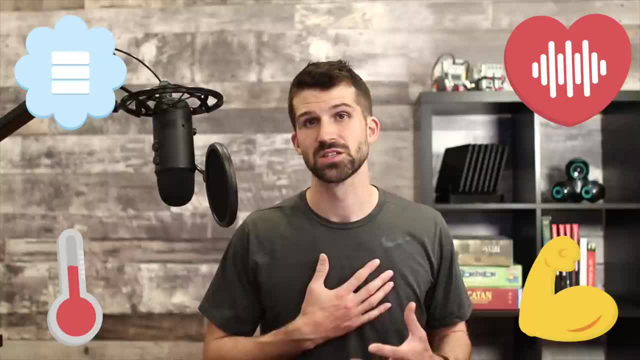 they feel warm. So take a minute just to notice all those things and pay attention to what your body's telling you. You got it, Okay. so what I want you to do right now is you're going to stand up And we're going to do a little. you choose fitness, So all you're going. 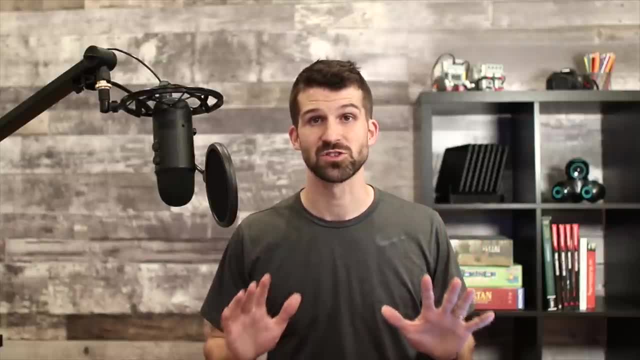 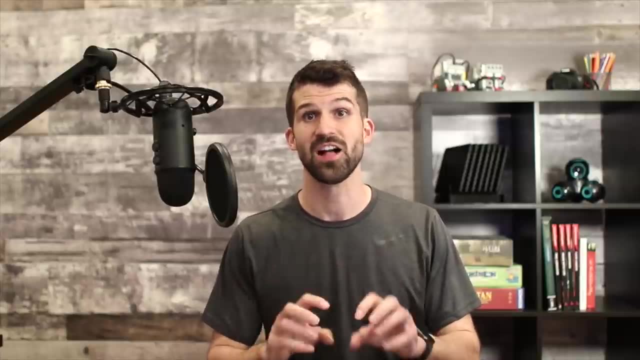 to do is I'm going to throw up on the screen. I'm going to put up two different exercises that are going to appear at once And you get to choose which one you want to do for 30 seconds. Your challenge is to try and go through all 30 seconds doing each exercise. 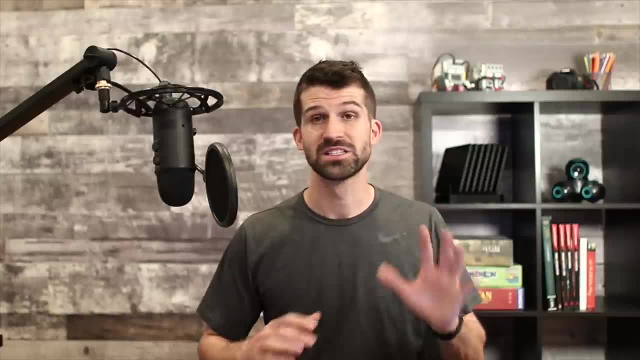 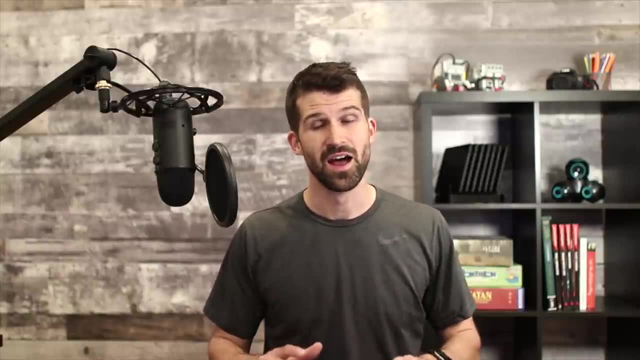 with the best technique that you can. After 30 seconds, you're going to see two new options And you'll get to choose from that. You're going to keep doing this until the end of the warm up And as soon as it's done, I want you to sit back down. crisscross applesauce. 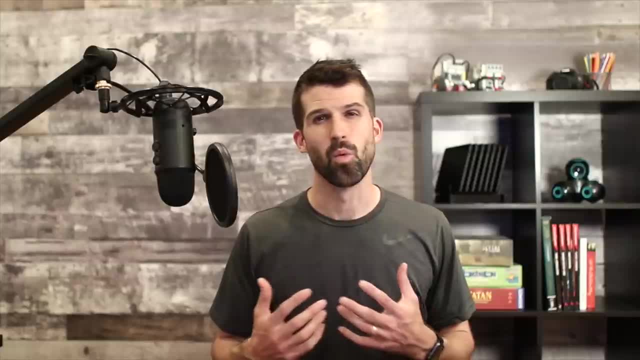 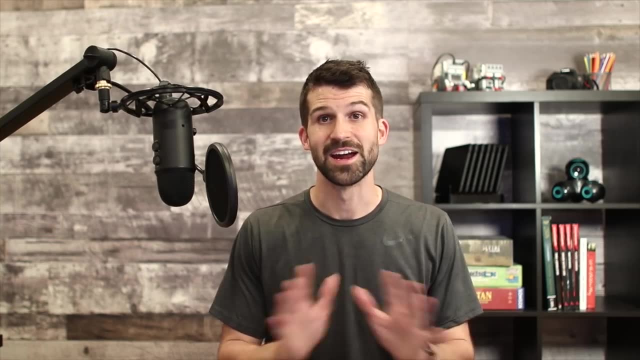 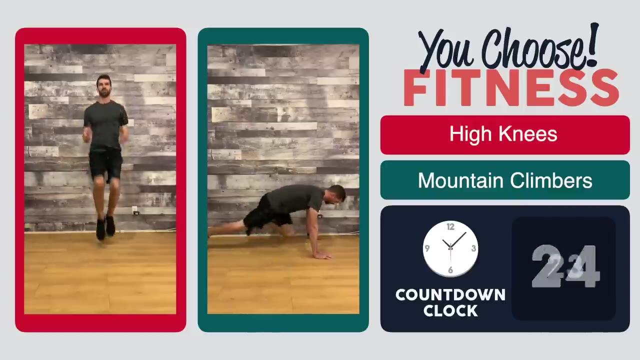 eyes closed, hand on your chest, And we're going to see what kind of changes happen in our body. Ready, Okay. so up on your feet. Ready, set, here we go. Okay, so you're going to sit back down. crisscross applesauce. 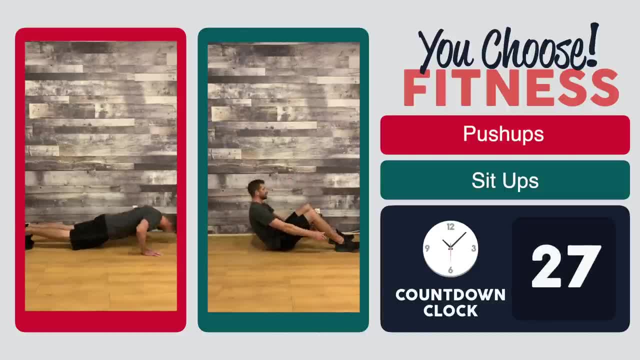 And we're going to reach the end of the warm up And when you do that, you're going to come back to the side and you're going to choose the right position. So you are going to sit back down and you're going to second you. 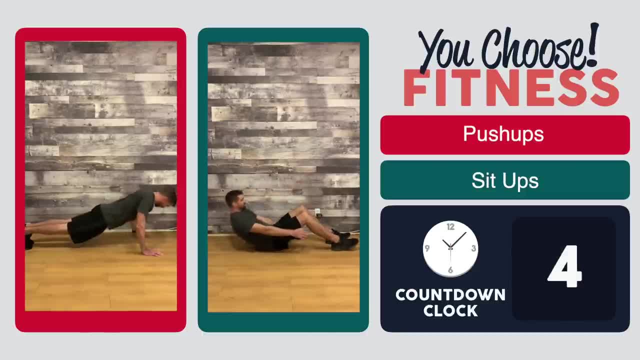 You're going to go up the spine and you're going to do a seat back up cross press. then you're going to sit down with your arms held together And once you're into that, you're going to step up and you're going to do a sit back. 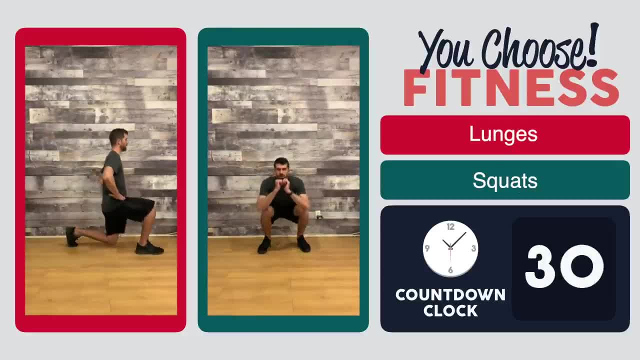 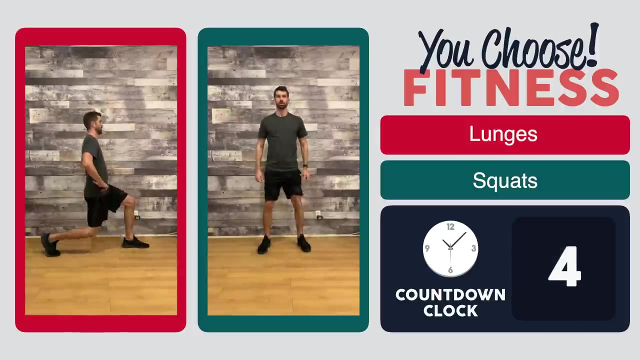 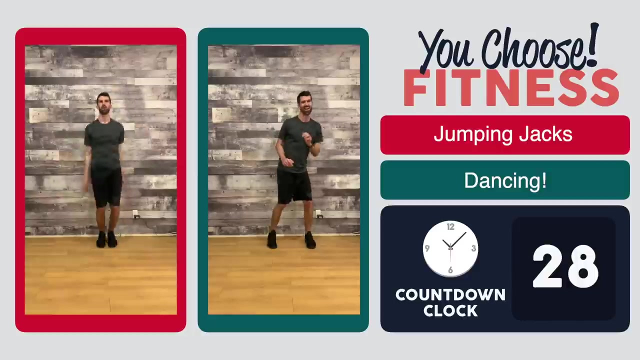 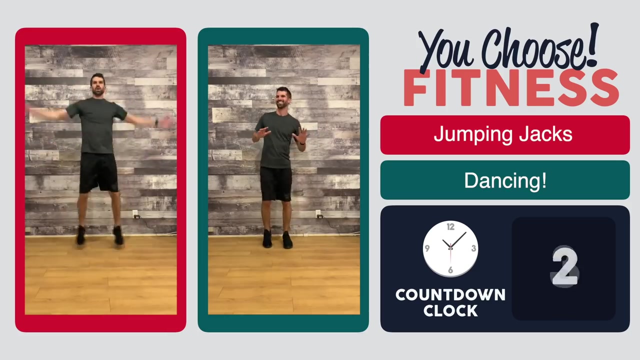 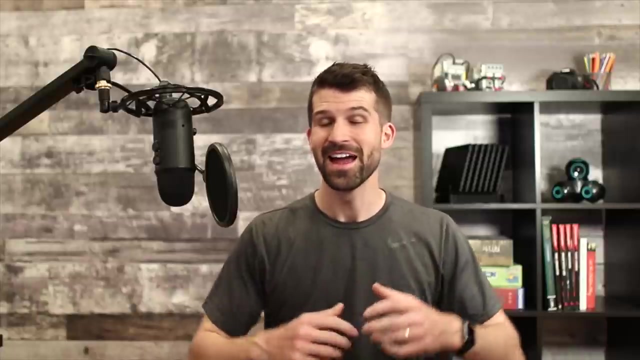 Thank you, Thank you, Wow. you were amazing Way to move and groove out there and get your sweat on. Okay, before we do anything else, though, sit down, crisscross applesauce, throw that hand back onto your chest. 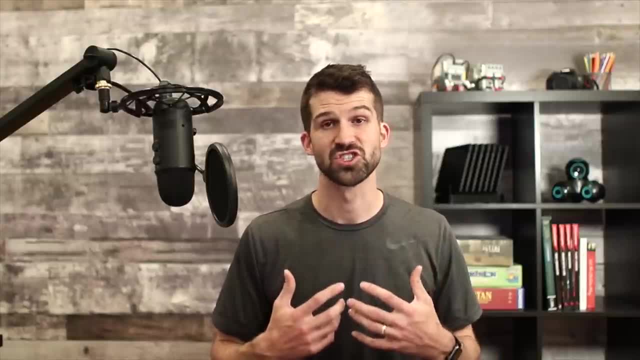 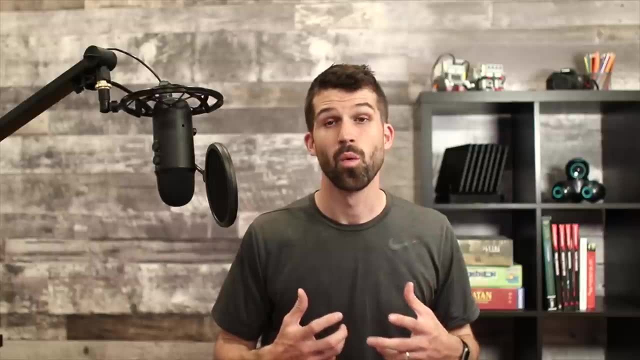 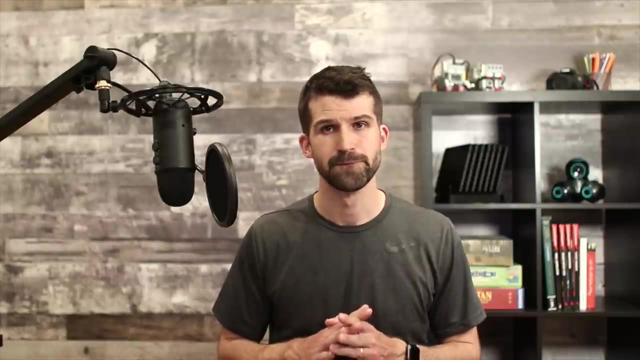 close those eyes and let's pay attention to what kind of changes just happen inside of our body. How is your breathing different than before you started exercising? What about your heartbeat? How about your body's temperature? Notice any changes there, And how are your muscles feeling? 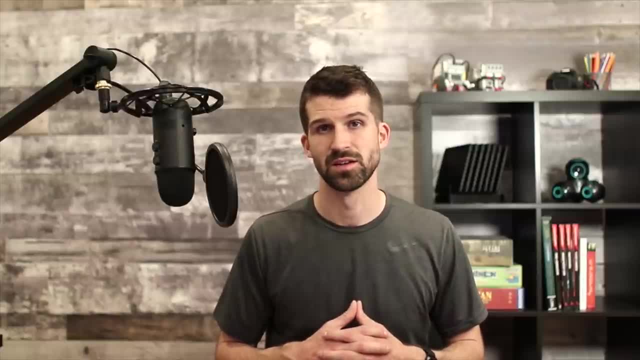 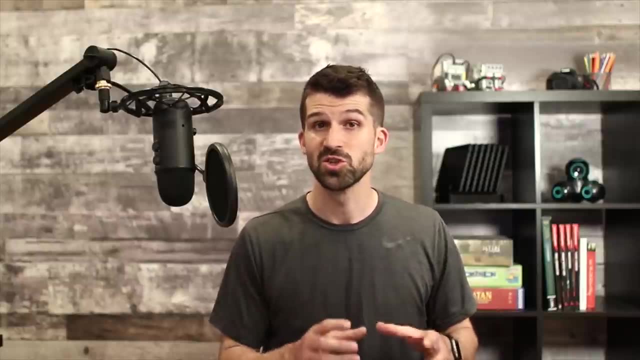 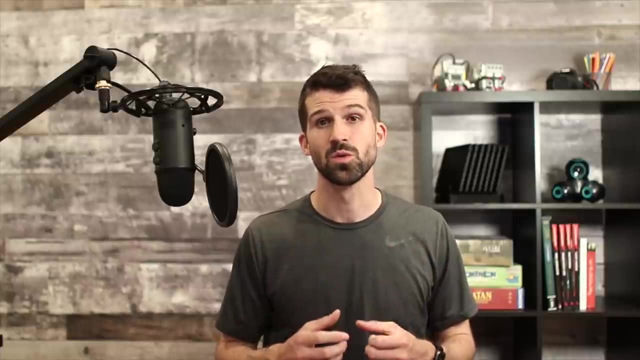 after all that exercise, all that moving, you just did See all those changes that you're noticing that just took place in your body. all those happens because you were physically active, And being physically active is one of the most important things you can do. 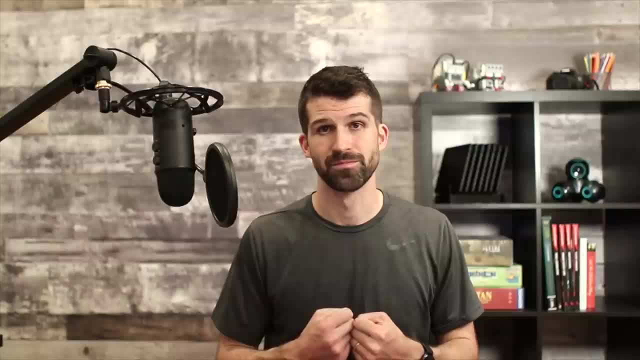 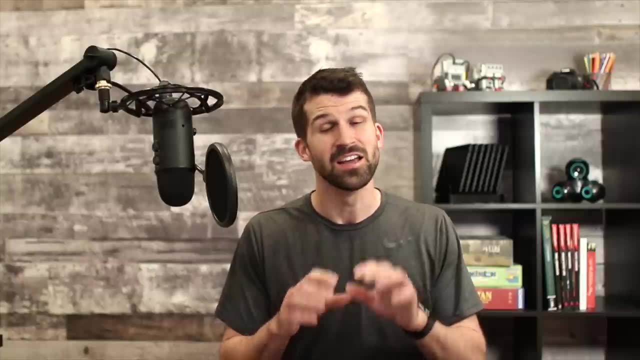 to try and keep your body healthy and strong. See, when you move, when you exercise, when you're physically active, your muscles break down in tiny, tiny, tiny, very safe kinds of ways And, in response to that, what your body's going to do. 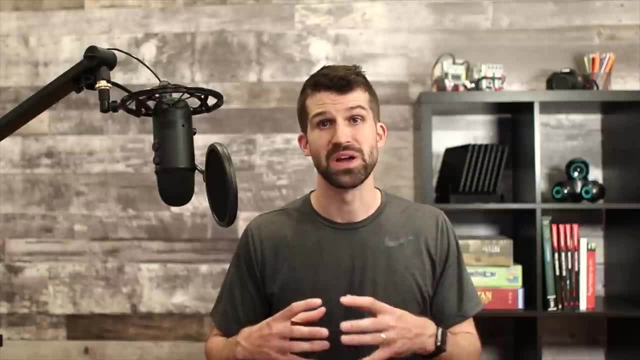 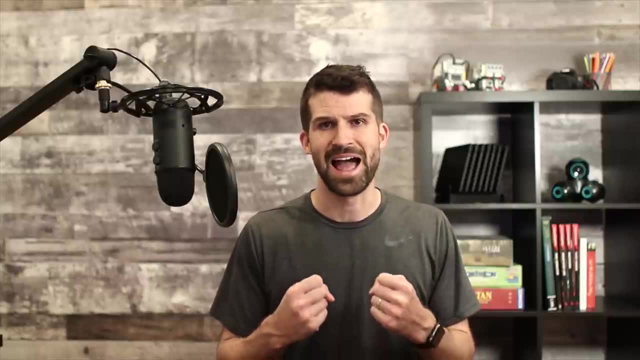 is. it's going to try to repair those muscles by making them bigger and stronger than they were before, so that the next time you do that kind of activity your body's more fit and able to handle all the different kinds of obstacles that you're trying to overcome. 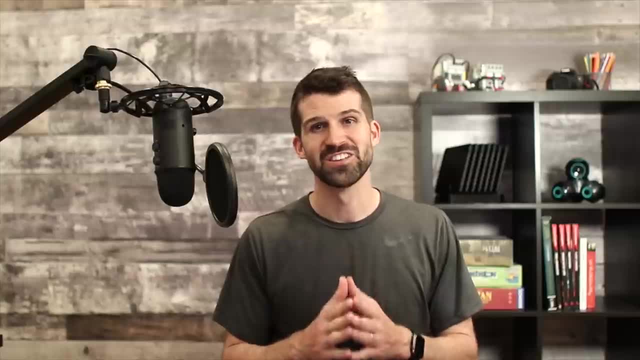 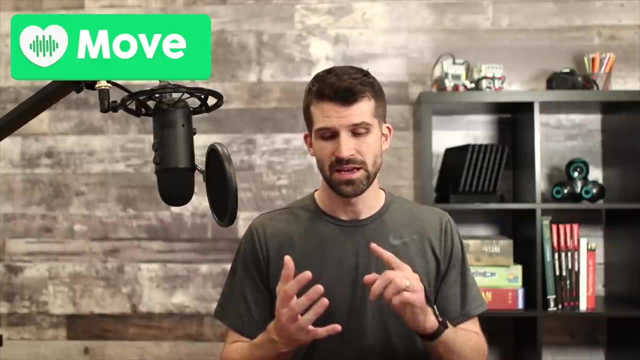 and all the resistance that you're dealing with, And that's why physical activity is one of the four important keys to physical health. The other three keys- eating, drinking water, getting lots of sleep- those are equally as important as physical activity. 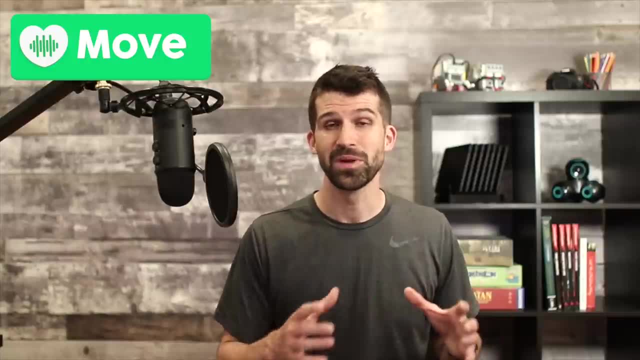 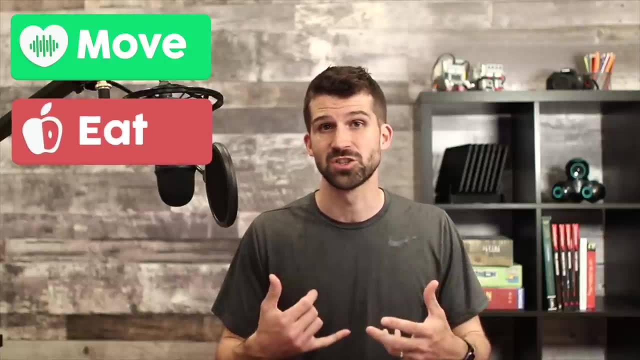 And they play a really key role in helping your body recover from all the exercise and all the moving that you do every day. Eating helps bring energy to your body that your body can use to be active, but it also helps deliver all the nutrients that your muscles and your bones need. 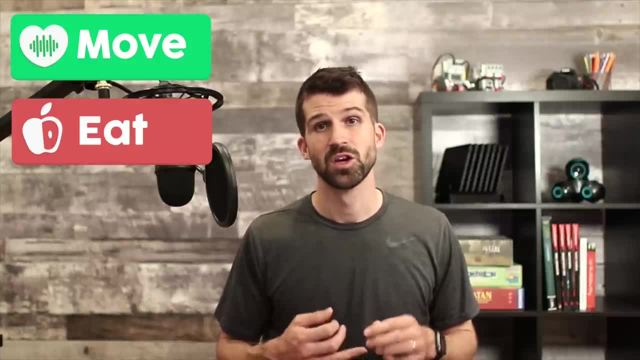 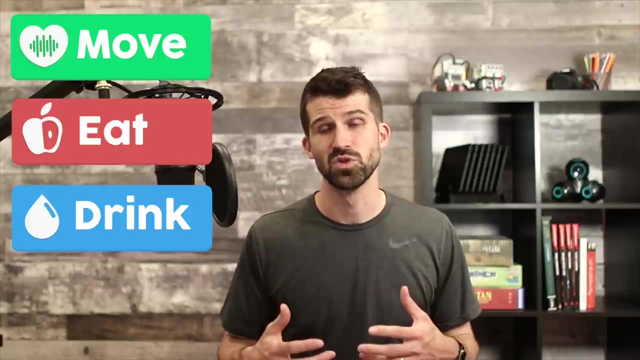 in order to recover from the exercise that you're doing. Drinking water helps your body run really smooth and can also help eliminate waste that your body produces as it's moving and exercising, And so sleeping gives your body the time that it needs to rest. 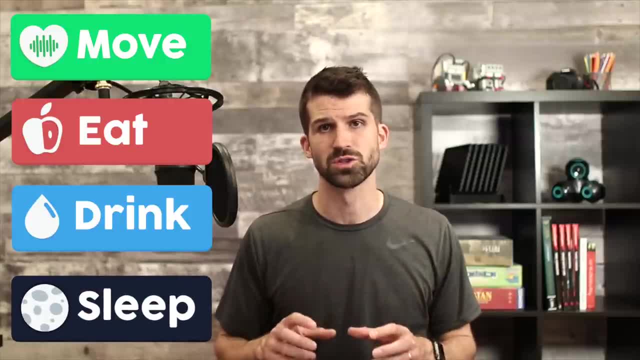 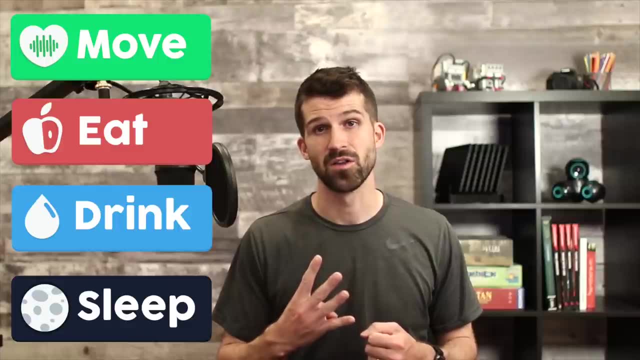 so that it can really focus on making all those repairs, so that you're growing stronger and stronger every day. So those are the four keys of physical health, And what I want to do next is knowing that physical activity is so important to keep your body healthy. 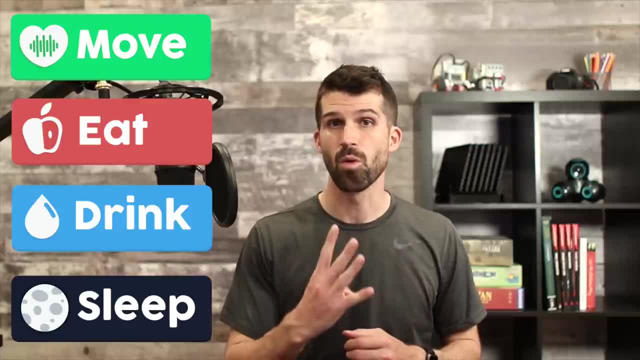 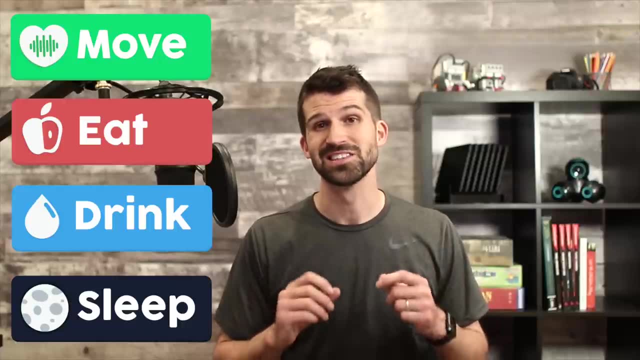 I want you to go out and try and find four different ways that you can be active at home while you're on this coronavirus break. so that you can be active at home, so that you can continue to stay healthy despite you not being at school and despite your whole world. 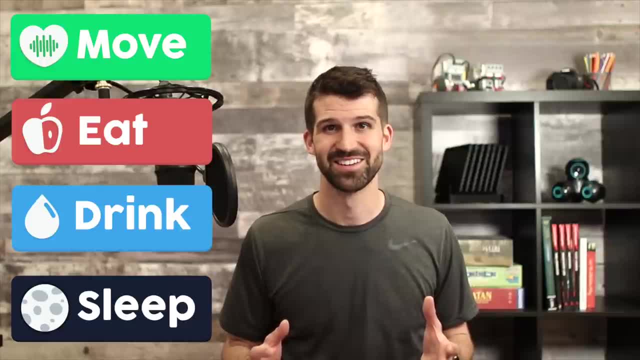 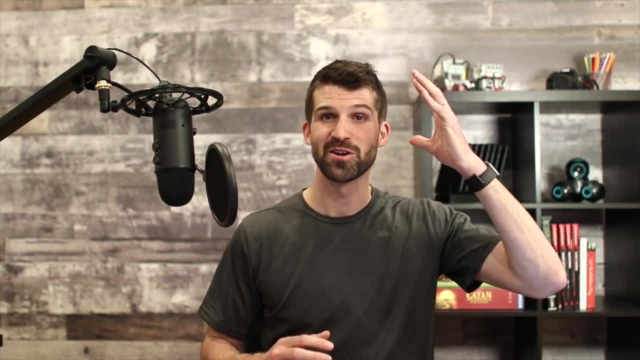 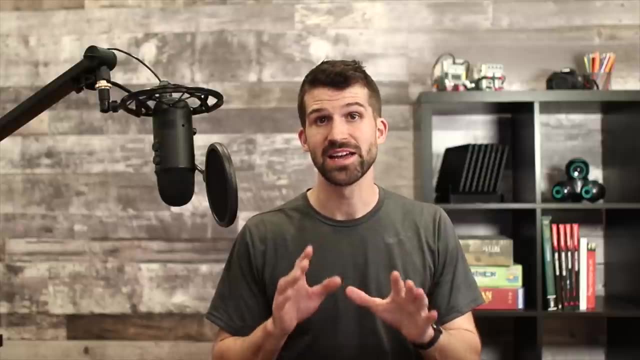 kind of being turned a little upside down. All right, so it's time to put on our Explorer hats, because we're going to go out and discover different ways of moving while we're at home. So your challenge right now, when I say go. 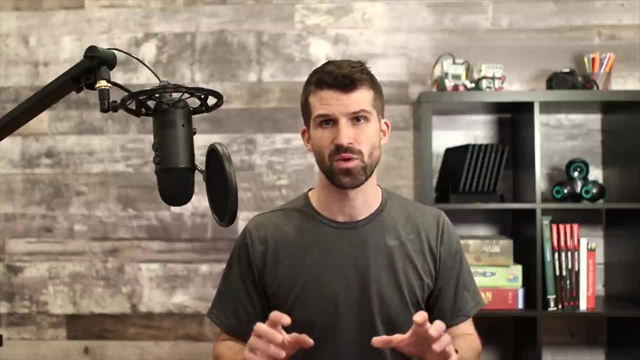 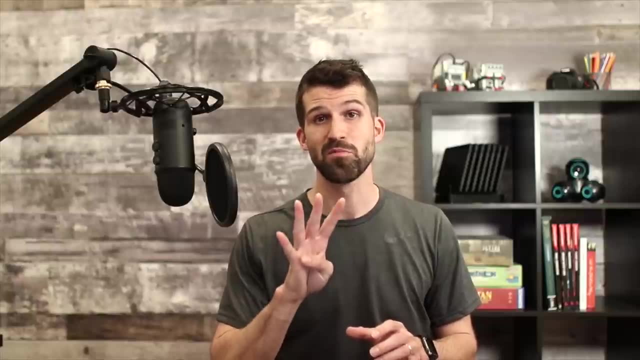 you're going to take off and you're going to go test all kinds of different ways of being active at home, And what you're looking for are four different ways that you can help keep your body healthy and strong by moving and grooving while you're at home. 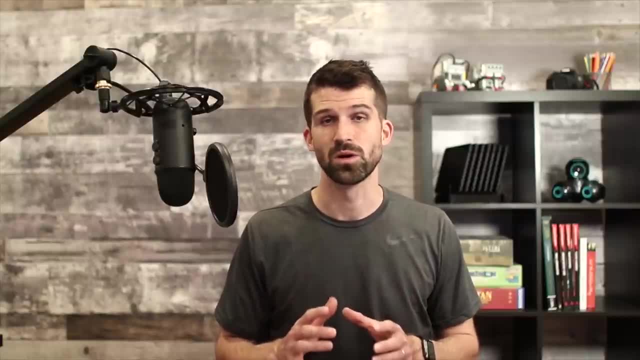 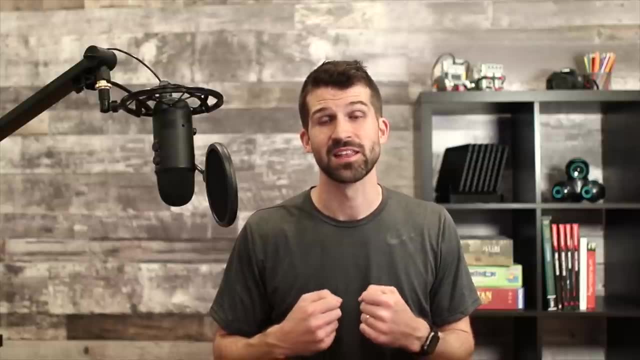 Now remember that not all physical activity is created equal. What you're looking for is physical activity that's going to really help your body grow stronger. The kind of physical activity is going to get the right kind of response from your body so that your body has to go. 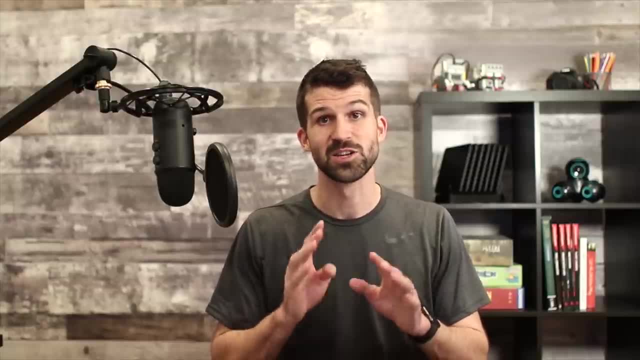 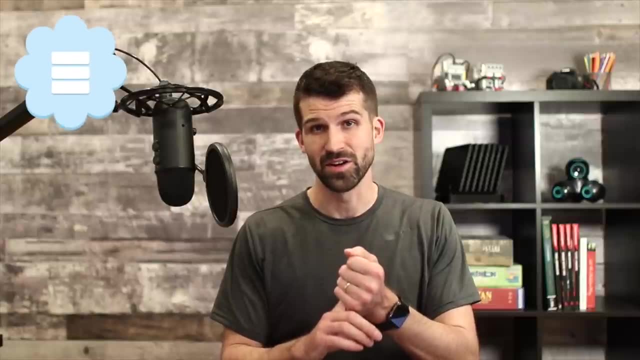 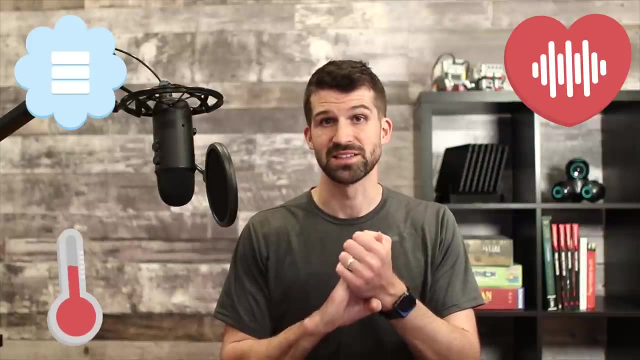 into that repair and grow mode. So if you want a hint, here's what you're looking for. There are four clues: You want to find activities that help make your breathing get heavier, your heart beat faster, your body gets sweaty and your muscles get tired. 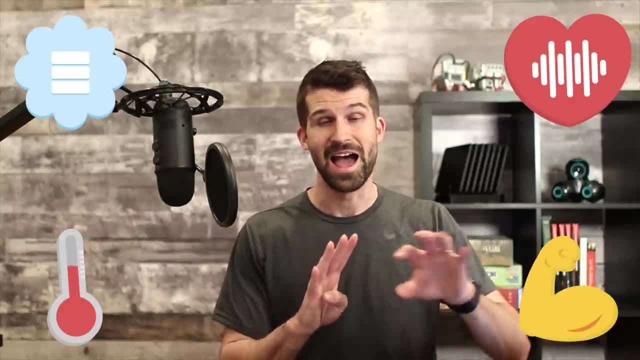 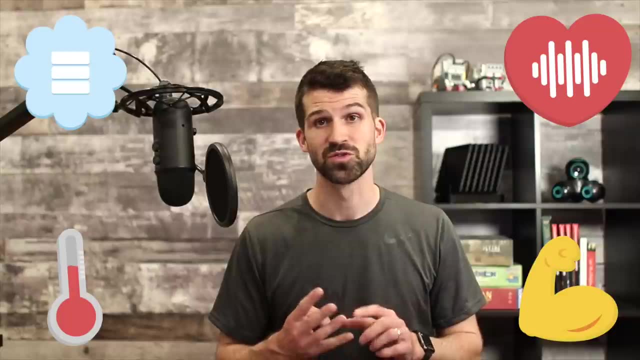 So those are the four clues that I'm going to be giving you And, as you go out and you test different ways of being active, check in and feel your body, see what's happening and see if you're noticing those four changes. 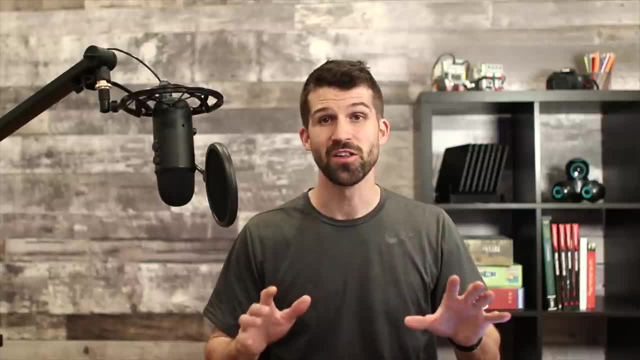 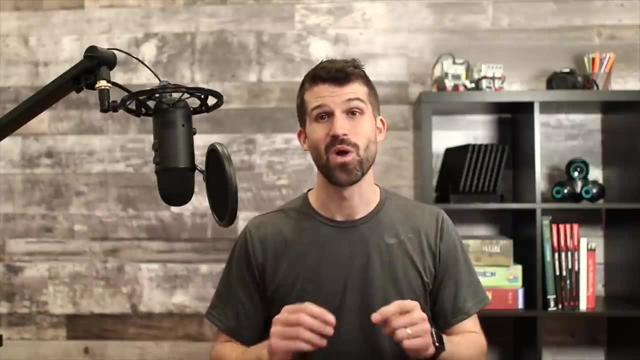 Okay, So you've got the information you need. You've got all the time you need. I want you to pause, pause this video, go out, explore, move, groove, do whatever you got to do, Okay, And when you have that list, 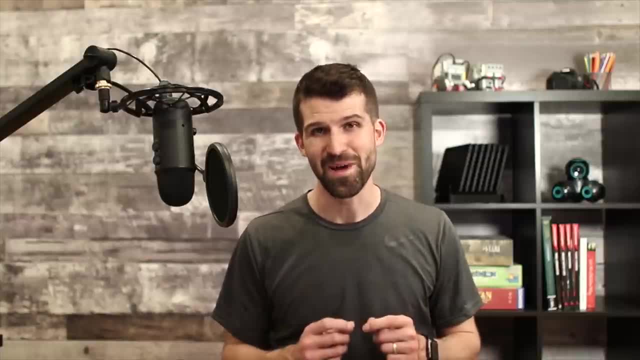 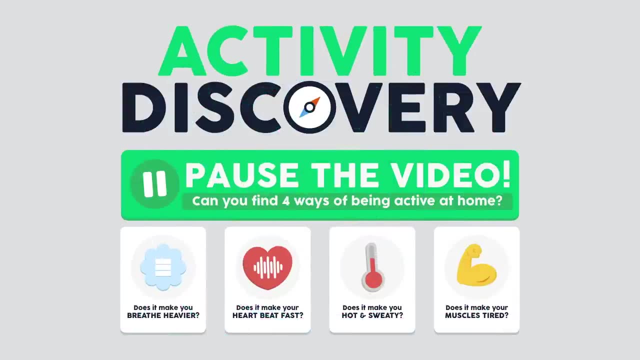 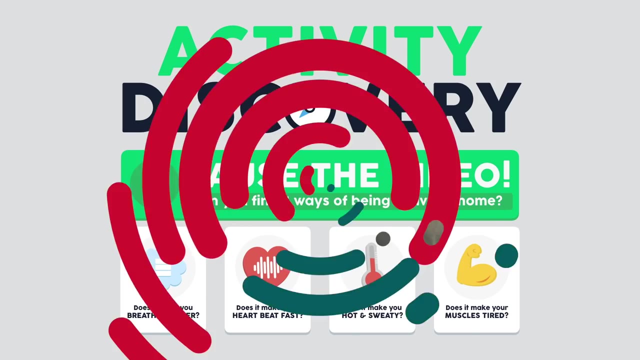 of four things that you know are the right kind of activities. come back here and we'll continue our lesson. Ready set go. Okay, welcome back. Did you find those four activities? Listen, I am dying to find out what you discovered. 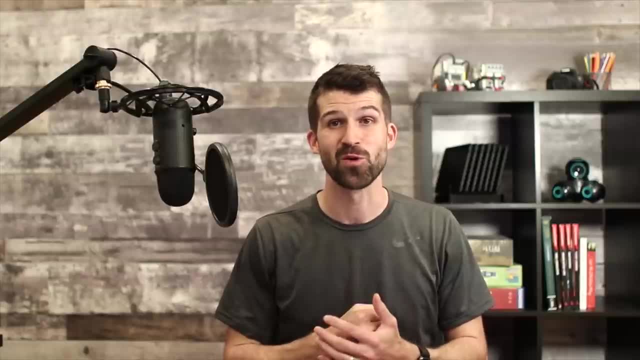 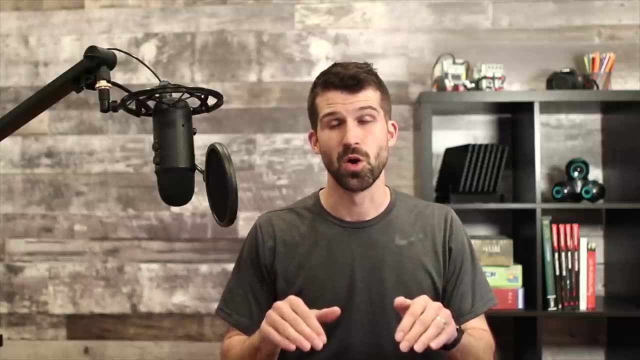 So what we're going to do now is we're going to create a happy heart power chart to try and showcase the four different ways of moving that you found. So in the description below you're going to see a link to that happy heart power chart printout. 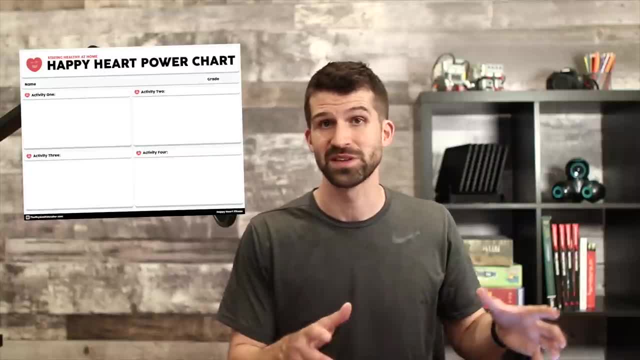 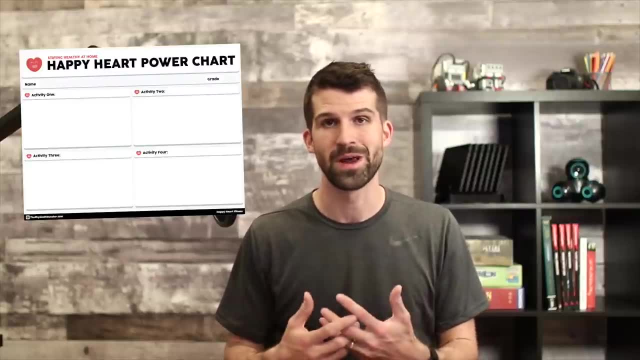 that I made for you And if you can feel free to go ahead and print that out now. But if you don't have access to a printer, do not worry. It is so easy to make your own happy heart power chart at home. 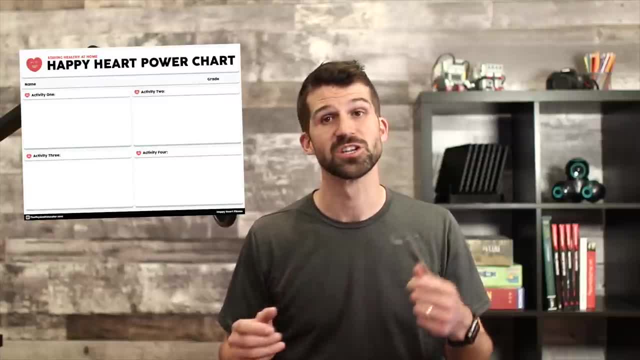 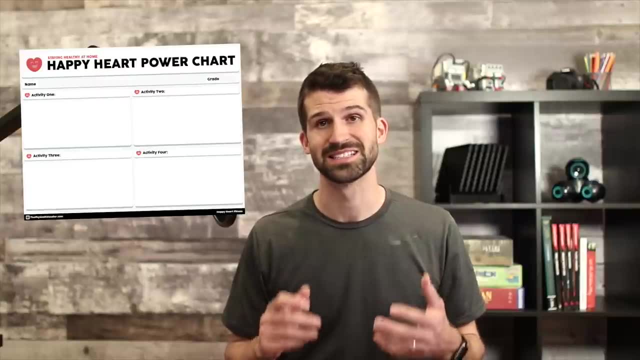 All you need is a blank piece of paper and a pen, And what you're going to do is you're going to take that sheet and you're going to create two lines that are going to divide the sheet into four sections, And you're going to use 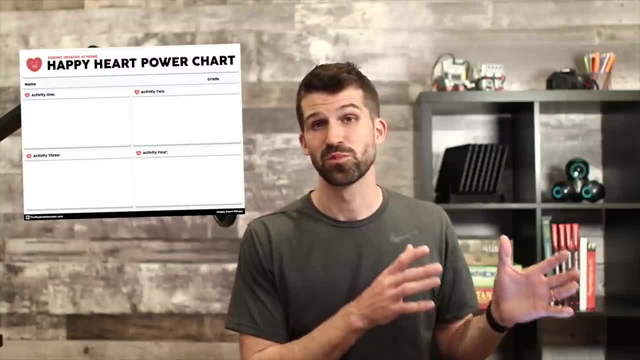 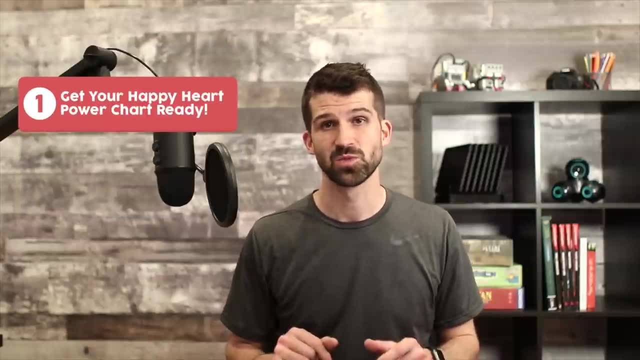 those four sections of paper, just like you would if you had printed out the happy heart health chart on your own. So once you have your sheet ready, you've printed it out or you've made it yourself. here's what I want you to do. 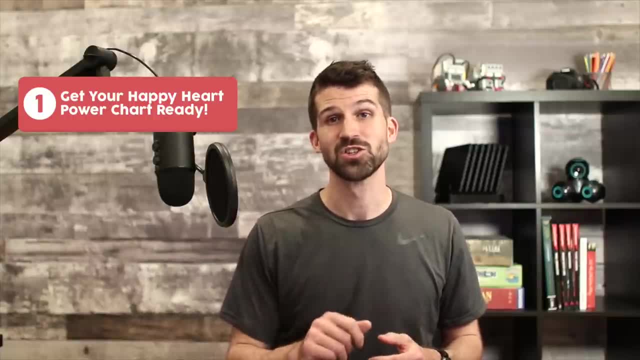 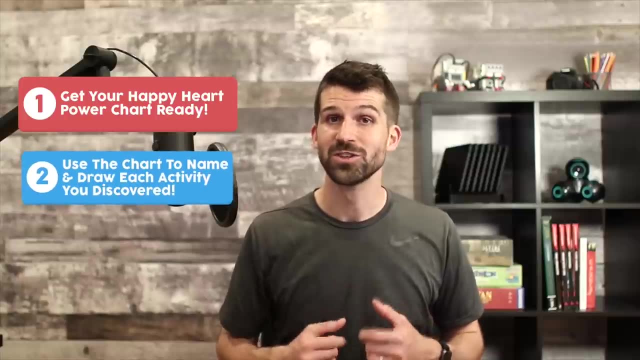 In each section of the document. I want you to write down at the top the name of the activity that you did as a title, And then, underneath that title, I want you to make a drawing of you being active in your house in the way that is going to. 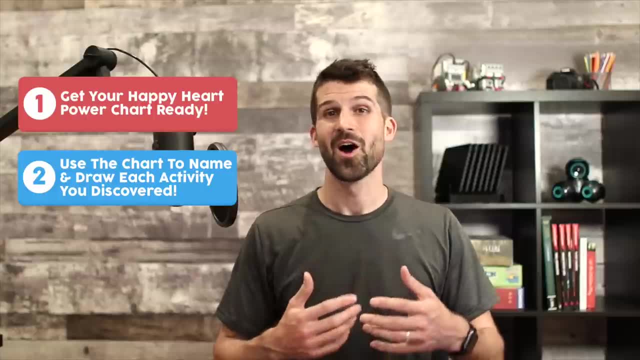 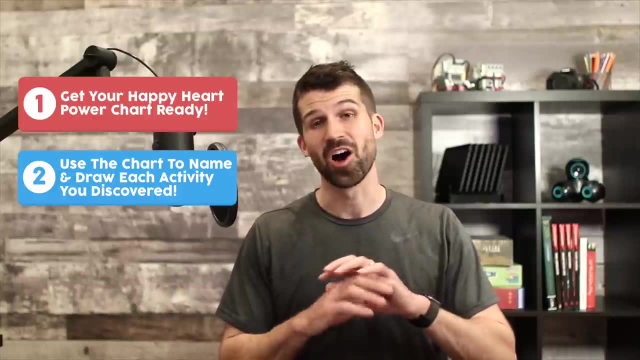 increase your breathing, get that heart beating all right. make you feel hotter, okay, get your sweat on and make your muscles start feeling tired. So take all the time that you need. You can take the rest of the day if you want. 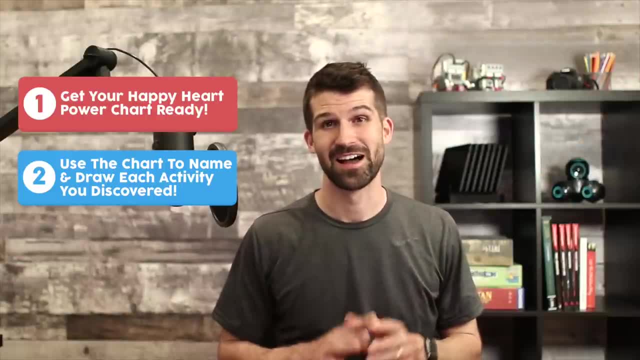 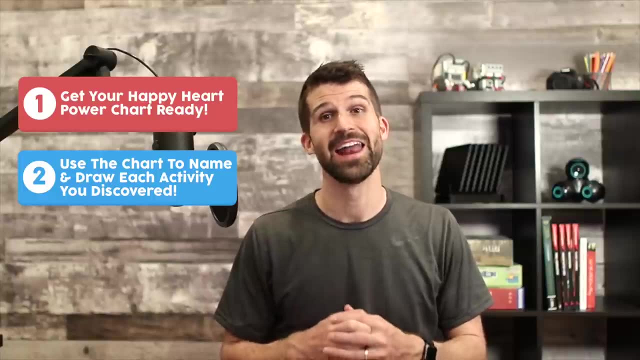 Take all the time you need to fill out that happy heart health chart And when you're done, when you have completed it, what I'd really encourage you to do is go ahead and share that with three people that you trust. The best way to do this right now. 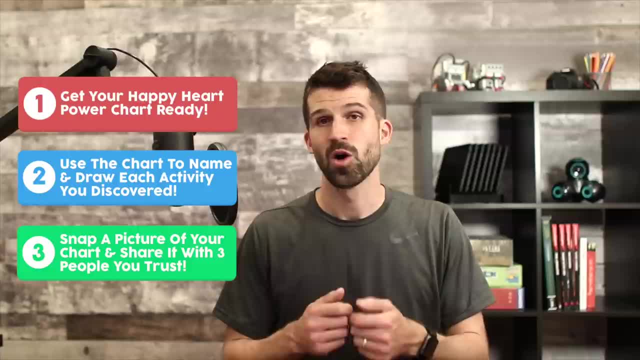 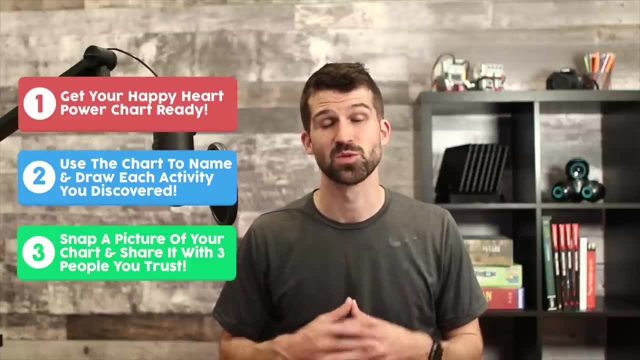 is to try and send them to it with iMessage or WhatsApp or whatever kind of messaging platform you're comfortable with or that your parents may have. And the reason I want you to share this with three people that you trust and care about is because we all need to be keeping active right now. 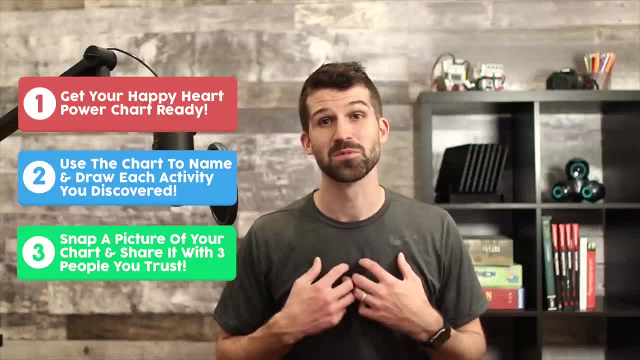 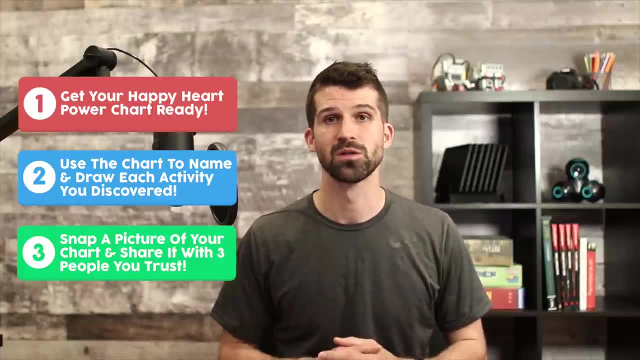 while we're at home during this coronavirus pandemic, and being able to have that time to have information shared between people who trust each other can go a long way in keeping the whole world moving. So, before we wrap up for today's lesson here, here's what I wanna do. 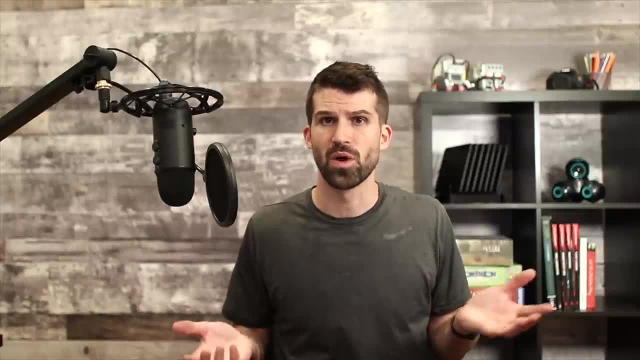 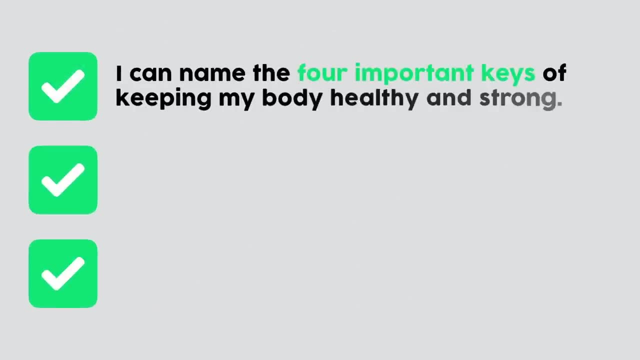 I wanna go back over our targets and I want us to reflect on whether or not today was a successful lesson. So let's take a look at those targets. So the first target says I can list the four important keys of keeping my body healthy and strong. 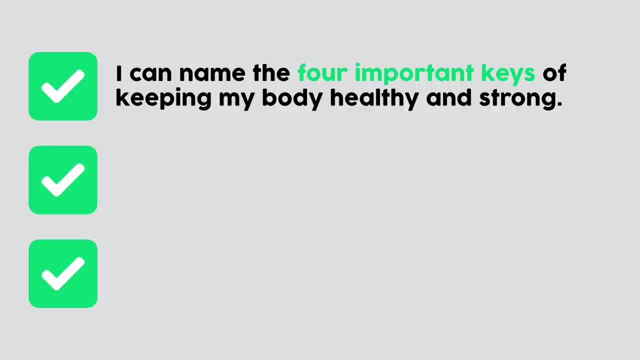 Do you know these? Try to name them all right now. The second target is: I can explain how physical activity helps my body stay healthy and strong. How does your body get stronger with exercise? Think about what we talked. what are the changes that happen inside your body? 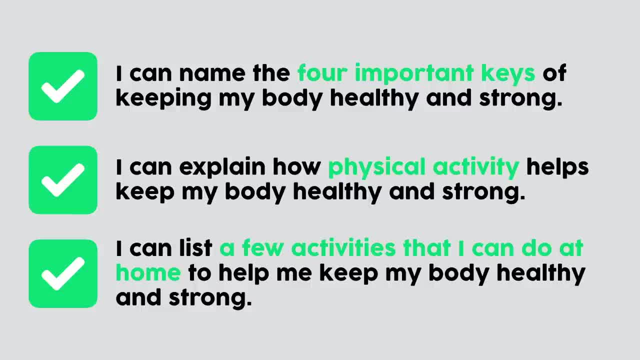 The third target was: I can list a few activities that I can do at home to help me keep my body healthy and strong. Check your happy heart power chart. You should have a few answers right there. right? So how do you feel about today's targets?